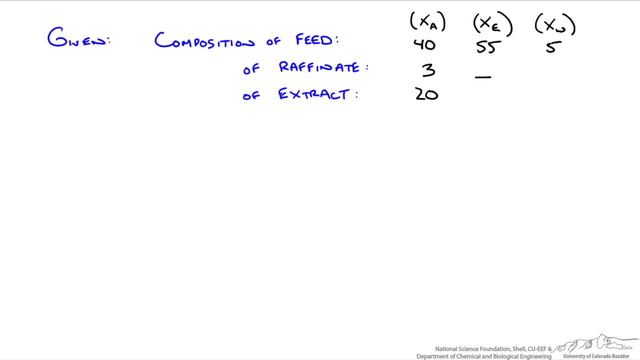 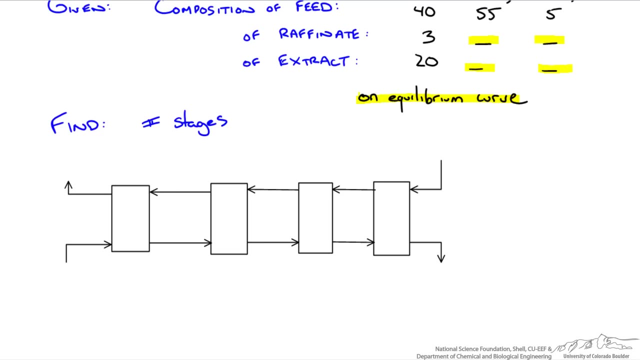 are assuming that in each stage we reach equilibrium, So these values right here will be on our equilibrium curve. So I have drawn a schematic here that represents our stages. Our feed enters at stage 1 and then we will go into stage 2 and what leaves stage 1 will be our raffinate. from 1.. We don't know how many stages we have, so we will have little n and our final, and we will have xn in each stage as well. So we know what the other combinations are. We are given a number of these values. We will name them, but we will use this as a reference. 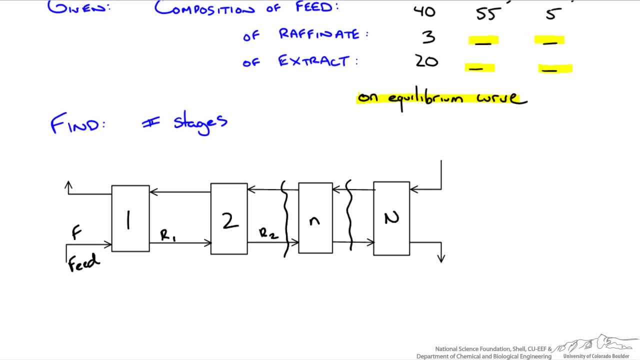 here And now we are going to see how this will look like. So we have a schematic here to represent our stages. Our feed enters at stage one and then we will go into stage 2 and what, and our final big N for the number of stages. So we know our raffinate leaving is going. 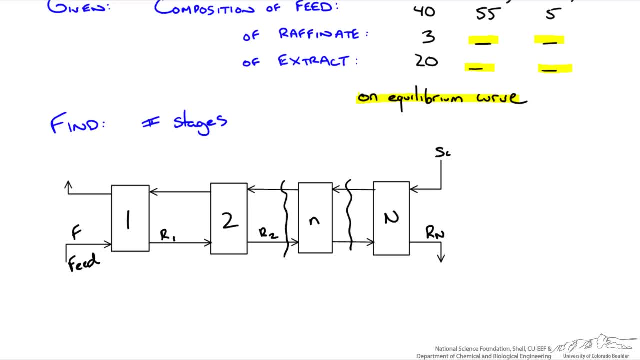 to be from the last stage. So for our counter current system, we are going to enter the solvent in here. We will say the solvent is S, So we have our extract leaving from stage N, our extract leaving stage 2, and our final extract leaving stage 1.. So we are going to 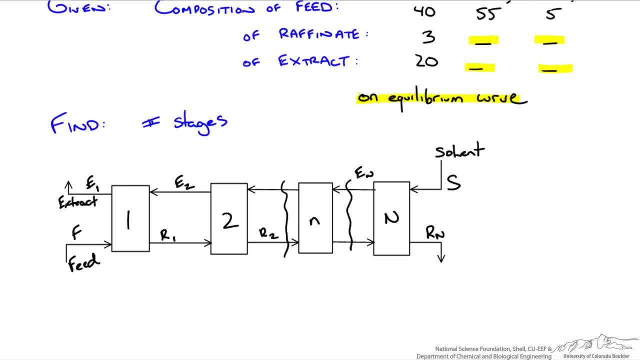 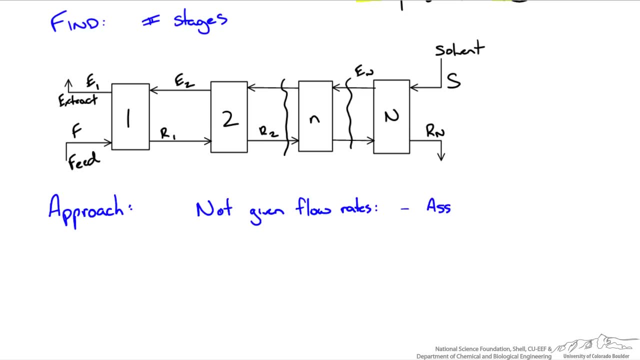 use this nomenclature as we move forward in solving our problem. We are not given flow rates, which means that we are probably going to have to assume a basis. We are also going to assume that the system operates isothermally, that any enthalpy associated with mixing is. 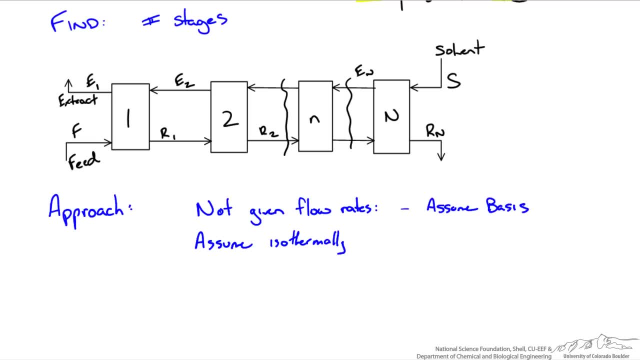 negligible, Since we are given our composition of our raffinate and our extract using the Hunter Nash method. we need to determine our solvent flow rate Once we have S. we are going to plot these points on our ternary diagram. We are going to plot our feed composition. 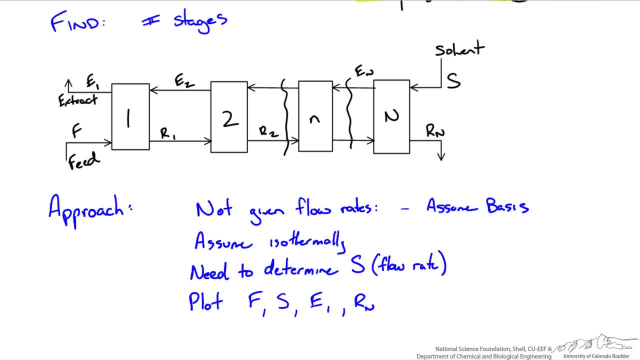 our solvent, our extract and our solvent. We are going to plot our feed composition, our extract, our raffinate leaving, and this all helps us calculate what is known as our mixture point. So let's start with step 1 and draw these compositions on our chart. 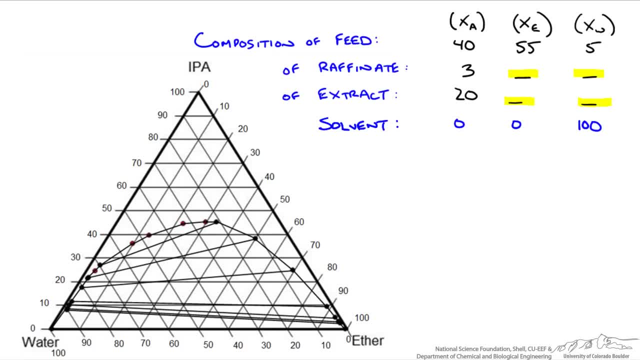 Since we are using a pure solvent, this is going to be all water. We can plot our feed by looking at 48% alcohol, and that is going to fall somewhere along this line. Then we can choose either of the other two points. So in this case, I am going to choose ether. We are going to go to 55%, which is going to be a lot of water. We are going to go to 50% water And we are going to go to 20%, which is going to be a lot of water. We are. 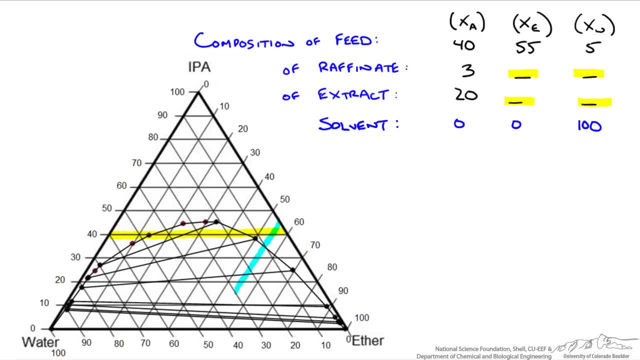 which is right between here, Where these intersect, gives us our composition of our feed. Now our solvent is pretty easy. We are going to use 100% water, So we are just going to draw a point over here. Now our extract and raffinate phases have to be at equilibrium, Not with. 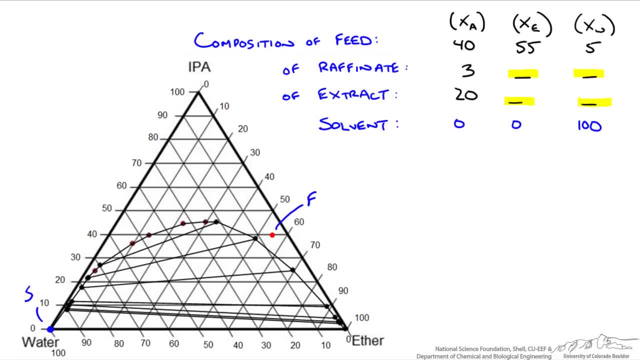 each other, but leaving the appropriate stages. So our extract has alcohol of 20%. So we know that is going to be closer to our solvent side. So we are going to look for where 20% of our alcohol is on our equilibrium curve. That is right. here We are going to do the 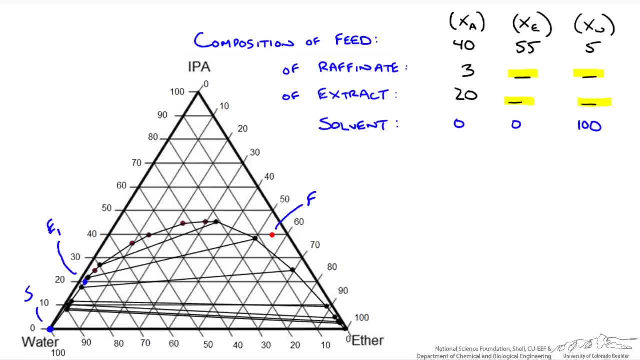 same thing for our raffinate. on the other side We are looking for about 3%, So somewhere around right here. So we have our four points Now. we could calculate the mixture point if we had flow rates for S and F. We know our feed enters our system with our solvent, So 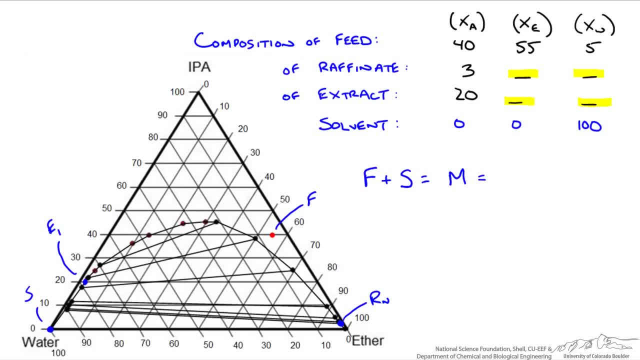 these two combine to create our mixture. This mixture also must be equal to what leaves the system, which is our extract And our raffinate. So we know that these three are on a line and these three are on a line. We get that by using a material balance and the derivation of why these points all fall. 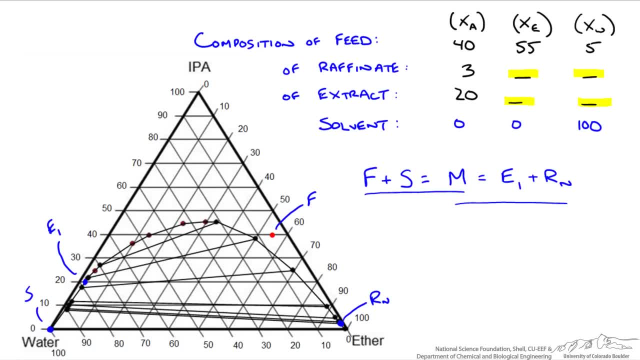 on the same line is shown in another video. So what we are going to do is draw a line from S to F and another line from our extract to our raffinate. Where these intersect is our mixture point. So now we could read the composition of our mixture point and use the 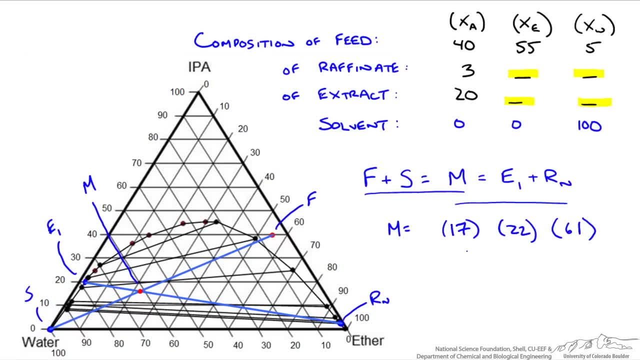 material balances to solve for a ratio of S to F. So this would give us an idea of how much solvent we would need per amount of feed to achieve this separation. Now, that wasn't asked in the problem statement, so we don't necessarily need to go down that road. But 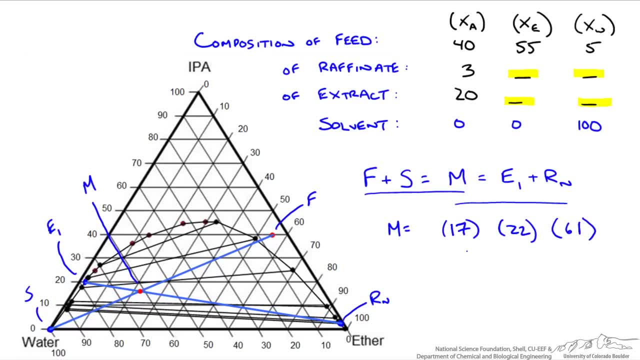 just to point out, the one thing we can do is use the inverse lever rule as well, Since we know that we could write S over F, equal to the length from M to F over the length from M to S, And this gives us about 1.48.. So we would need almost 1.5 times more solvent. 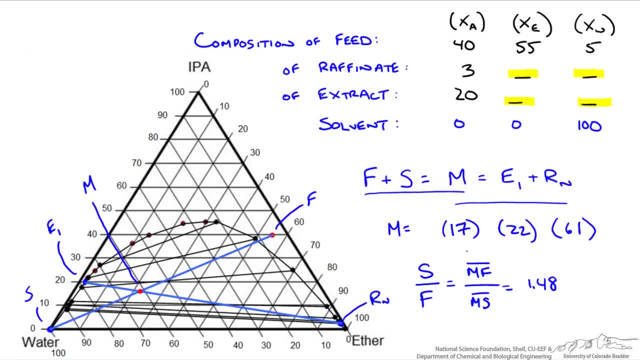 than our feed to achieve the given compositions that we are proposing Now. we could also use the inverse lever rule for our extract and raffinate, since we can then calculate the ratio between those two And, using what we know from our feed and solvent, performing. 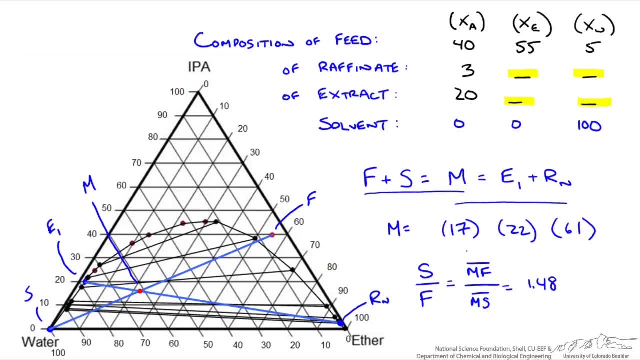 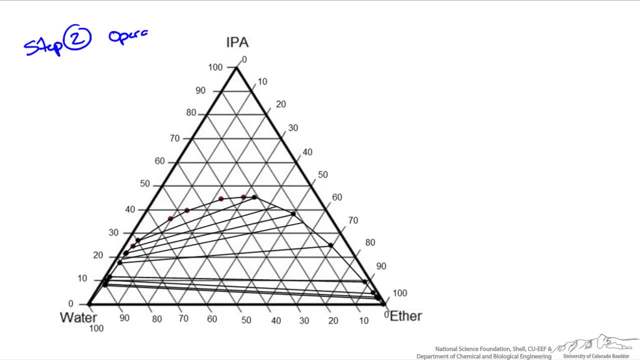 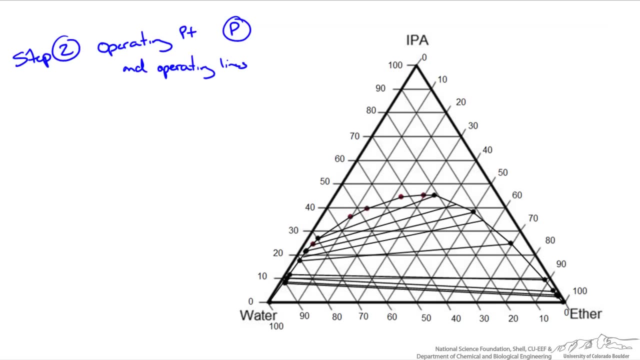 our material balances gives us an idea of the absolute amounts of these two phases. So step three, Step two in this process is to determine our operating point. We're going to say it's called P here And our operating lines. So what we're looking for is a point P. So point P is a. 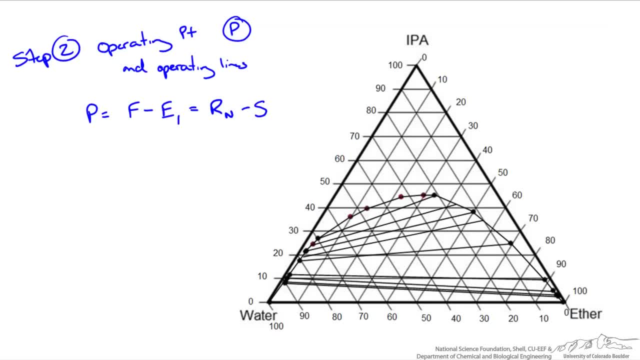 solution to our material balances, and we know that these must be on a line as well as those points. So we could draw these two lines going through our points. So we'll start with our line that goes from F through E1.. And we'll draw another line that goes between Rn and S, Where these 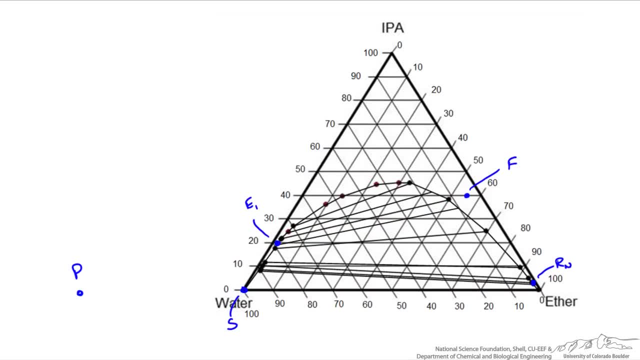 intersect is going to be our point P. So the last step, step three, is to use our tie lines and equilibrium lines to determine the amount of stages that we need. So we have our operating point and we know that each line that goes through this point is going to include the passing streams And what I mean by that. let's take a look again. Let's end with a number of passes, So we know that each line that goes through this point is going to include the passing streams And what I mean by that. let's take a look again. 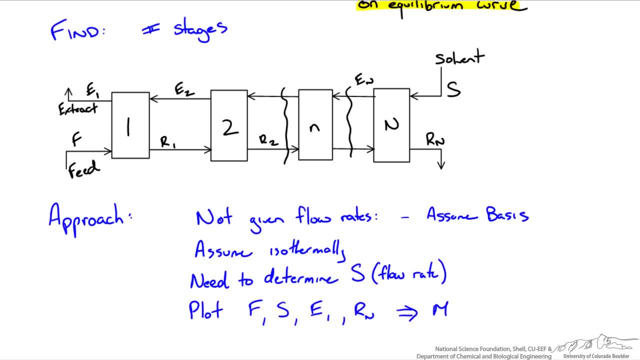 And what I mean by that. let's take a look again at our schematic. We know the difference between this stream and this stream is the same as the difference between this stream and this stream, and that difference is p. So that also means that E2 and R1 fall on a line with p, and En and Rn-1 would fall on a line with. 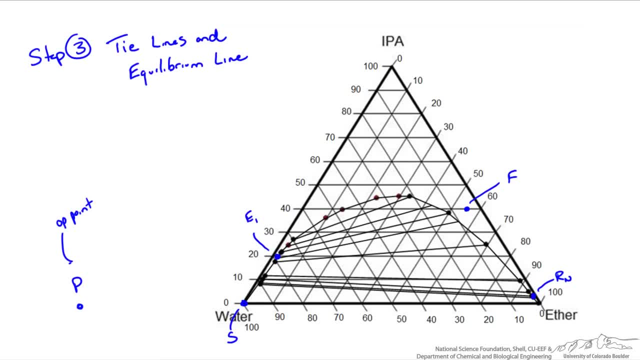 p. So the first thing we do from stage 1 at E1 is to follow the tie line, since we know at stage 1 we're going to get equilibrium, So we follow that tie line to the other side. So I draw a point on the equilibrium curve on the other side for our raffinate and I'll 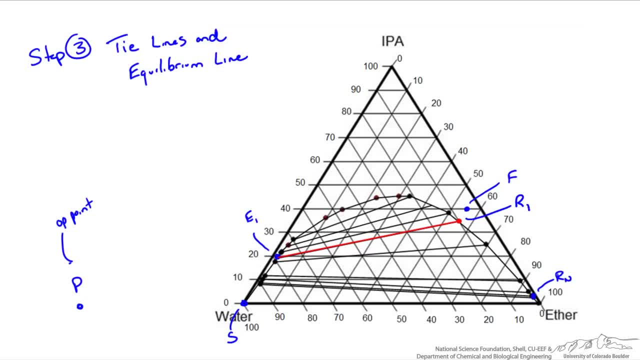 label that R1.. So we know that R1 and E2 are passing streams that fall on a line with p. So we'll draw a line from p to R1 and where it intersects on our equilibrium curve is going to be where E2 is. 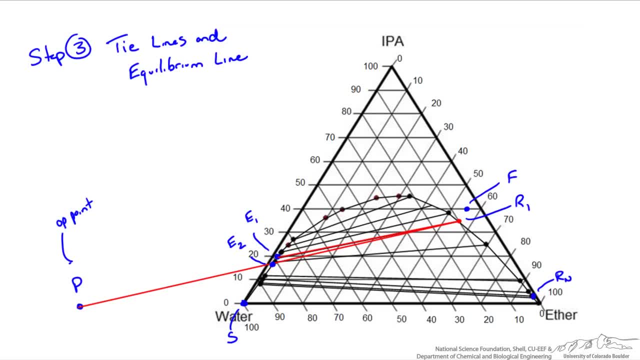 So then from here here we repeat the process of following the tie line from E2 to the other side where we think R2 is going to be. Now I had to interpolate here, so that's probably my best guess, without doing our interpolation method, to draw more tie lines. So again we know R2 and E3 fall.